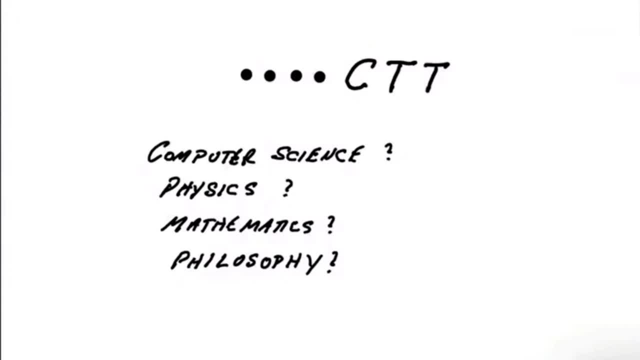 some sense they're all of them. But whatever it is, they are what they are And they form a kind of interesting set of guidelines for thinking about the connection between information, between computer science and physics, And I think there's a great deal of value in exploring the connections. 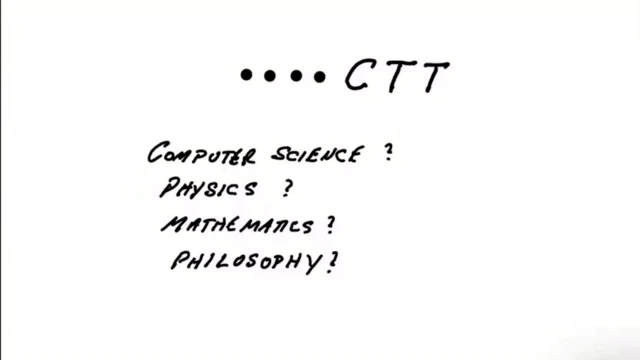 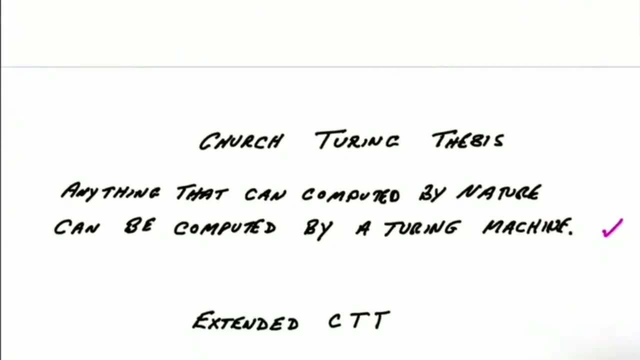 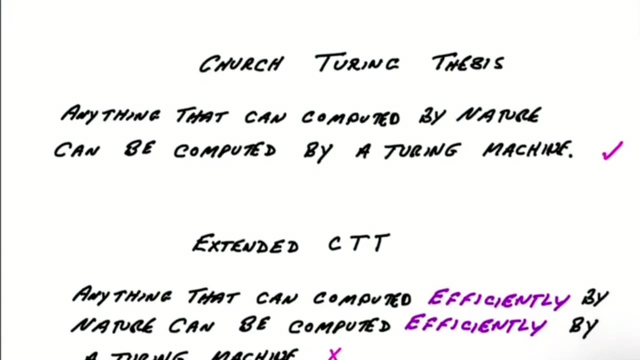 even if the precise version of these theses is not completely well known- And I think it's not true, It's not completely well known. But let's begin. Let's let me just outline. what are the various theses that we're talking about. There's the original Church-Turing thesis, Anything that. 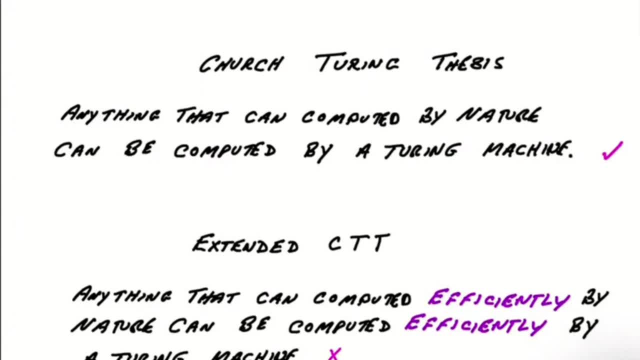 can be computed by nature can be computed by a Turing machine. I'm not at all sure this is the way either of those people said it, But that's what it comes down to. Anything that can be computed by a natural process can be computed by a Turing machine. This idea is closely connected to Wigner's. 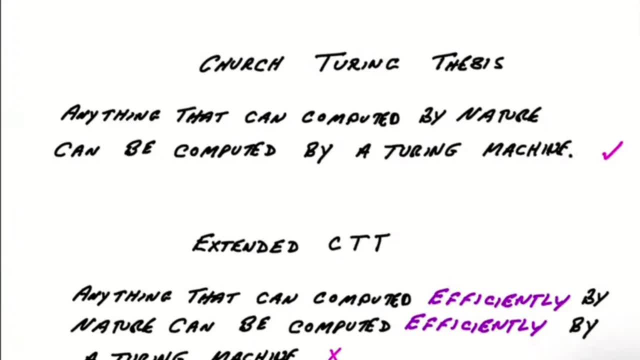 puzzling question: what is it that makes mathematics so effective in studying the laws of nature? And the answer is, of course, the laws of nature are mathematical. Well, if mathematics is, by definition, computation, not all mathematicians will agree that it is computation. 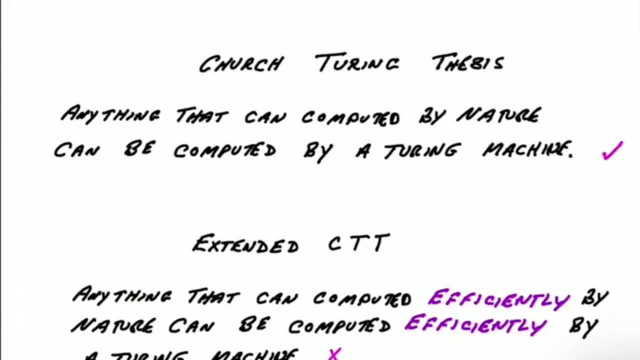 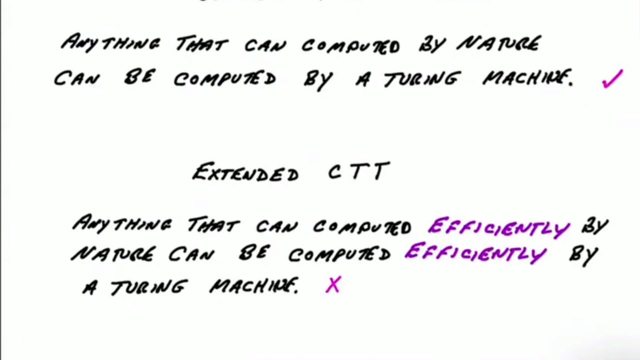 But at least some mathematicians would consider mathematics to be basically computation And the laws of physics are mathematically mathematical, then it pretty much follows That anything that can be computed by nature can be computed by a Turing machine. So is it true? I think it's true. Is it interesting? I think it's interesting. Is it a tautology? 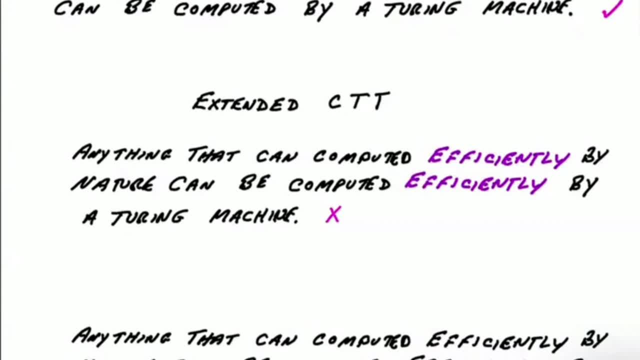 Maybe, but it's one of these interesting tautologies. Next we come to the extended Church-Turing thesis: Anything that can be computed efficiently- efficiently, I take the mean in less than exponential time or less than exponential number of steps- 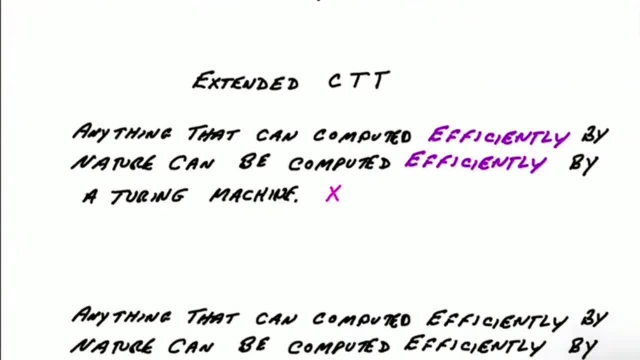 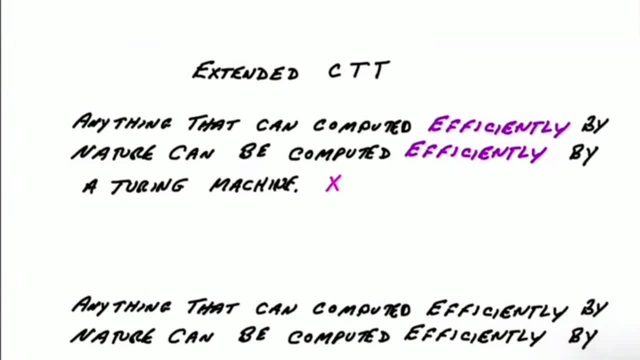 anything, perhaps a polynomial number of steps, anything that can be computed efficiently by nature can be computed efficiently by a Turing machine. Now, this is a very interesting example, because it's known to be false, or at least believed to be false. There's nothing like 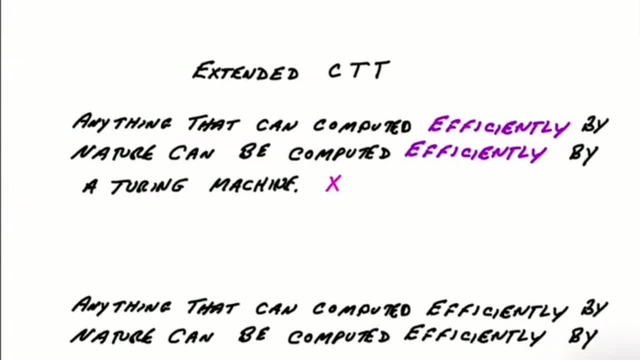 having something which turns out to be false, to convince yourself that it had some, that it actually had some meaning and that it can be refuted. Why is it false? It's false because we think that quantum computers can compute things that could not be, or that quantum 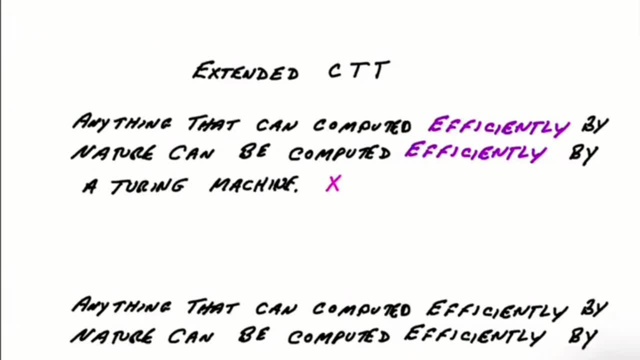 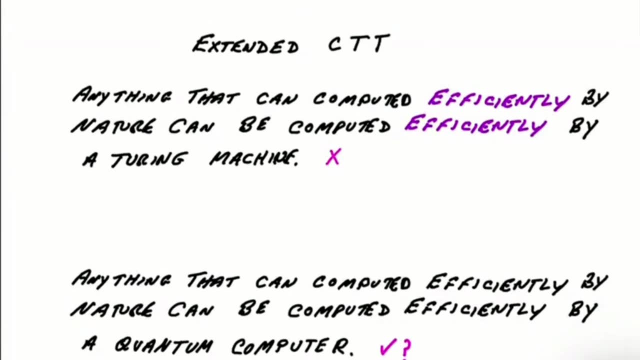 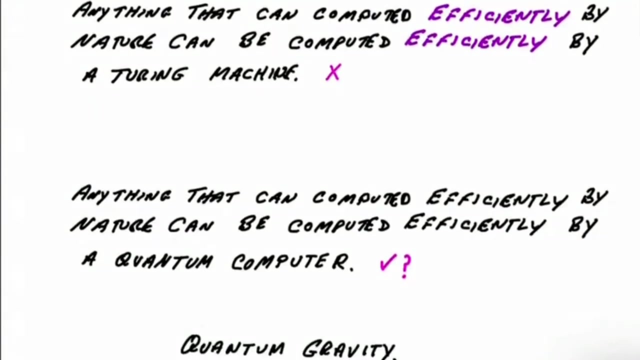 mechanics. because of quantum mechanics, nature can compute things efficiently. that Turing machine could, not a classical Turing machine. That led to what is called the quantum-extended Church-Turing thesis, and that was a simple elevation of the idea from classical physics to quantum mechanics, and it said that anything that can be computed efficiently by nature 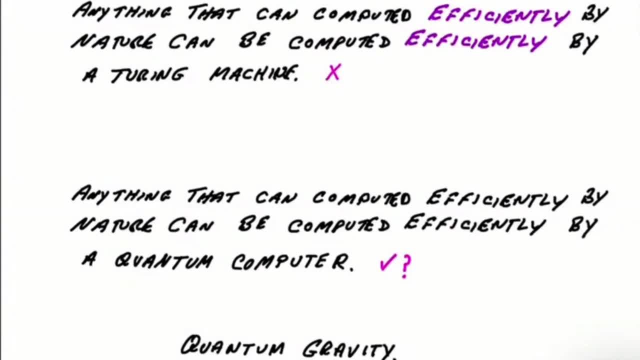 can be computed efficiently by a quantum computer. Now, is this true? Most, I think, people would say yes, most people, most people never heard of it. but most probably people in the audience here would say, yes, it's true, probably true. I have one question about it. 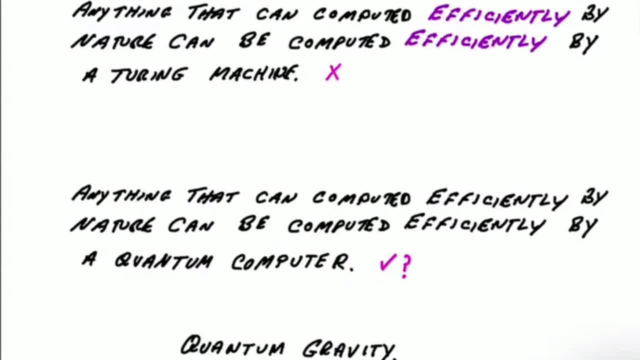 It's not so obvious to me that quantum field theory, because of all of it's infinities and because of all of it's subtleties, cannot in principle compute things which could not be computed by a quantum computer, by a conventional quantum computer. It comes down to the question of whether a quantum field theory can be. 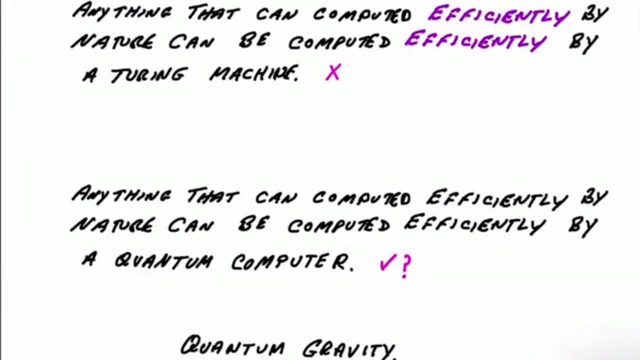 simulated by qubits. If a quantum field theory really cannot be cumulated, can be simulated, then you might wonder whether the quantum field theory can do things that a system of qubits can't. but I'm going to leave that out now. I'm not going to get into that. 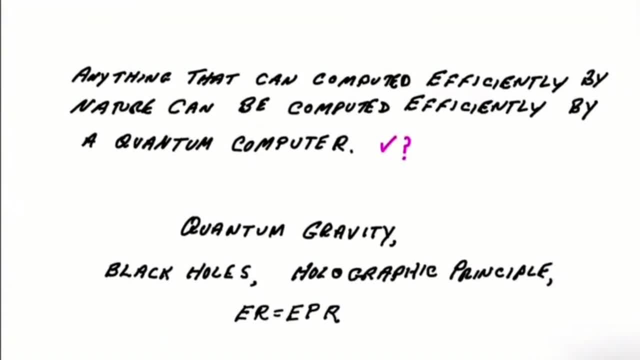 although I think it is an interesting question. Can an arbitrary quantum field theory be quantum simulated by a system of qubits? Okay, but we're now undergoing a paradigm shift. In fact, I would say that we can judge the revolutionary character of a paradigm shift. 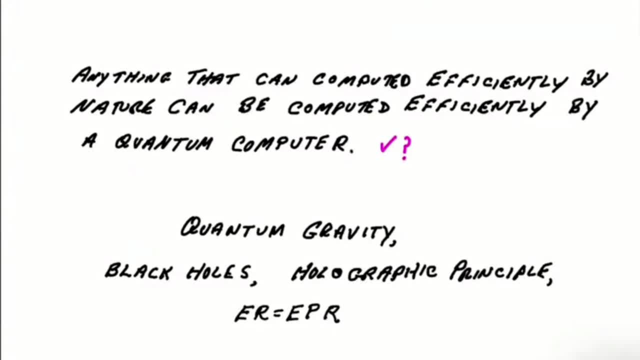 in physics, by how much it makes us rethink the Church-Turing theses. and we are undergoing a paradigm shift in physics now- The quantum gravity shift. it's full of surprising ideas like that: the horizon area is equal to entropy, the holographic principle.